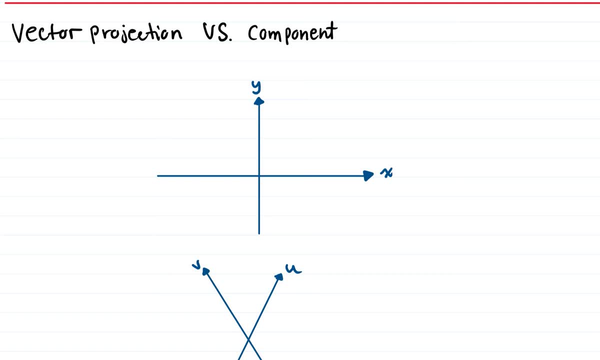 Hi, In this video we will discuss the difference between vector projection and vector component. Lots of students, when they start studying engineering statics, they get confused by the difference between vector projection and vector component. The best way to explain the difference between them is using two examples. 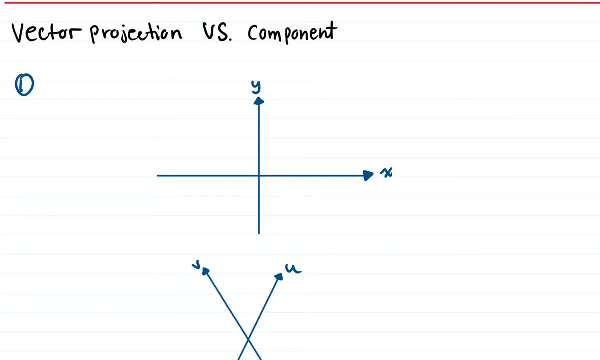 So let's discuss the first example, The first one. we have x and y-axis. These two axes are perpendicular to each other. They form a 90-degree angle between x-axis and y-axis. Okay, so let's draw from the origin a vector. 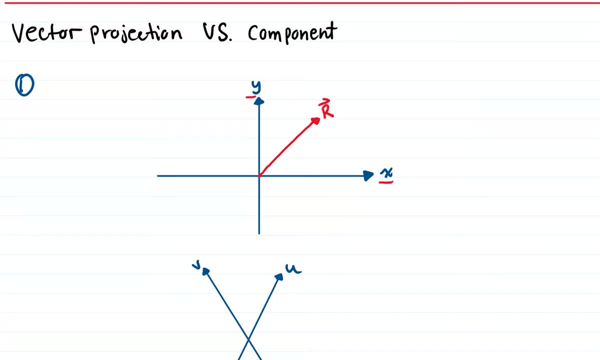 Let's call this vector r. Let's call this vector r If we want to, If we want to do the vector projection. projection means a shadow of the vector on the x-axis or the y-axis. So if you imagine that we have a light in here, 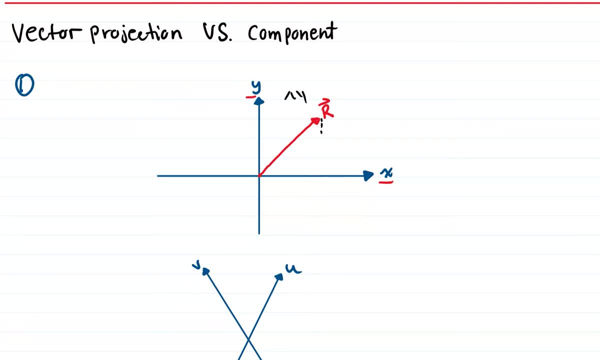 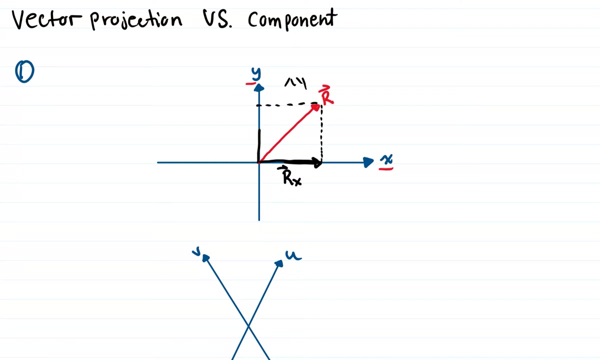 that light will create a shadow. So what we are drawing, What we are drawing now, is the shadow of vector r. This vector, we will call it rx. We will also create another shadow on the y-axis and we will call this ry vector. 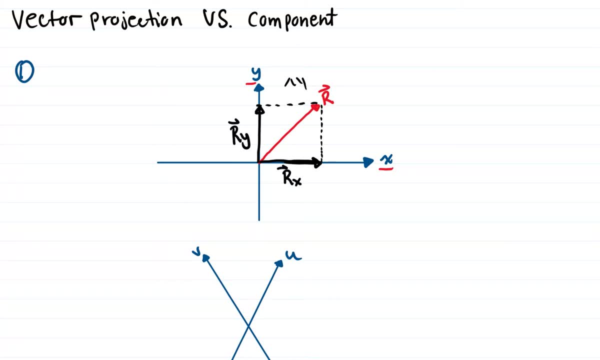 Alright. So now, Now we know that these two are vector projection, Are these two vectors rx and ry are also vector components. The word components indicates addition, So if we added rx plus ry and they give us vector r, that means these two vectors are. 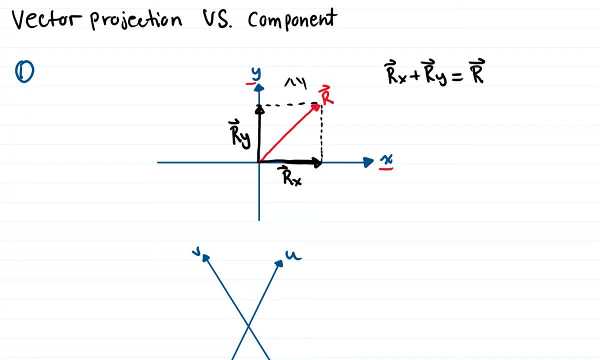 vector components. So if we use the head to tail fashion and added rx to ry, where we gonna place the tail of ry to the head of rx and draw ry with the same length and direction. so when we added these two vectors they give us the resultant vector r. 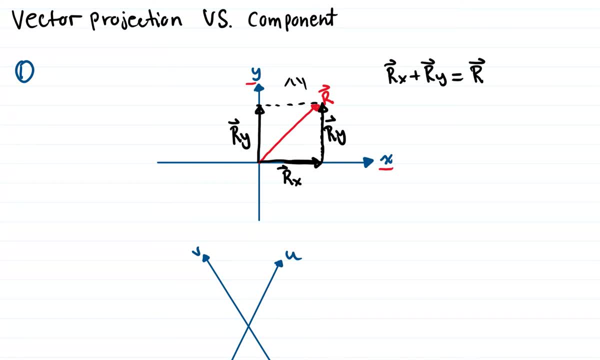 So these two vectors, rx and ry, are vector projection and vector component. So when we want to find rx, we can say r cosine theta, let's say the angle between them is theta. If we want to find ry, we can say r times sine theta. 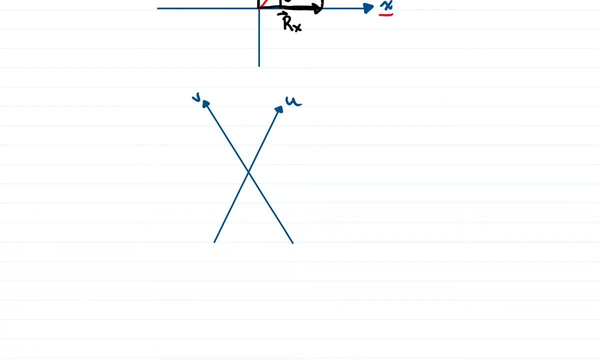 Now let's go to the. For example in here we have u and v axis. These two axis are not perpendicular, They do not form a 90 degree angle. So let's draw a vector in here. Let's call this vector f. 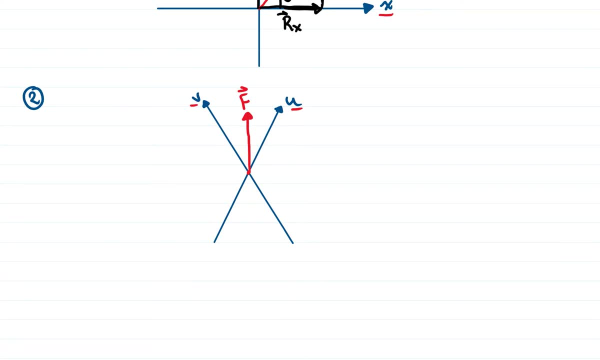 Let's draw a vector in here. Let's call this vector f. Let's draw a vector in here. Let's call this vector f. And now we are gonna draw the vector projection which is the shadow of vector F on axis u or v. 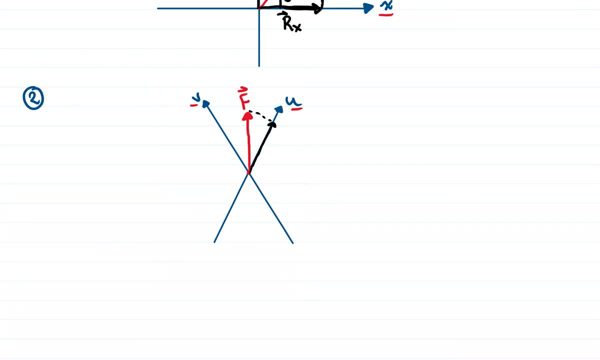 So this is fu projection vector on the u axis. Cool, Now let's create another projection. Let's work on the same object on the v-axis. so this fv projection vector. now, are these two that? so now we we know that these two vectors are vector projections. are these two vectors are also vector component, as we mentioned? 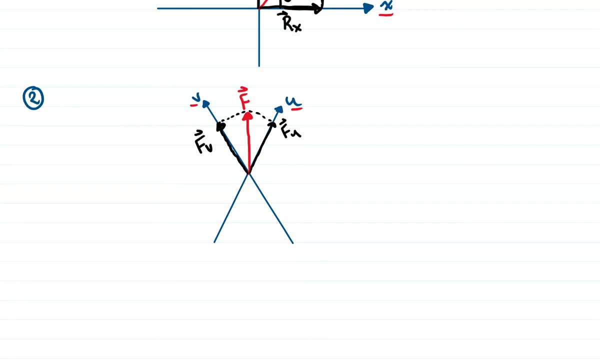 in the beginning component mean is if that if we added these two vectors, they will give us vector F. if we add these two vectors using head-to-tail fashion, will they give us vector F? the answer is no, because if, if we can take vector F and place it still on the head of vector F, you 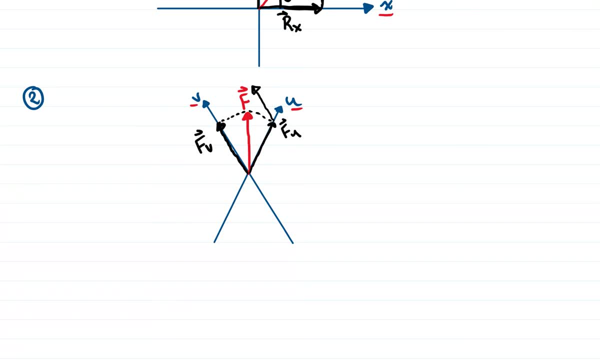 it won't give us vector F, all right. so how can we find, in this situation, the vector component of the vector F and the vector function of the vector function of the vector function of component? so the best thing you can do is to draw a parallel line to each axis where these 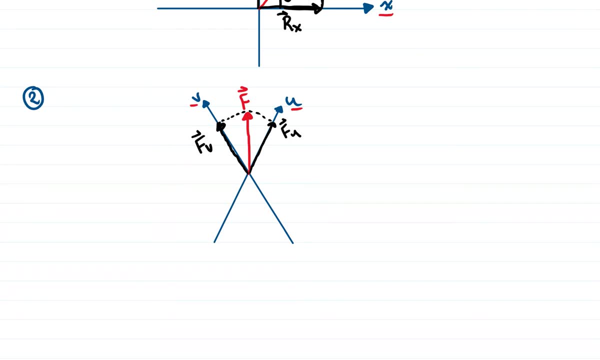 two lines will intersect at the head of vector F, meaning: so this is the v-axis. so now let's draw a parallel line to the v-axis and let's draw another parallel line to the u-axis. this way, so this vector in in green, if you is called the vector component, and this vector F, V in. 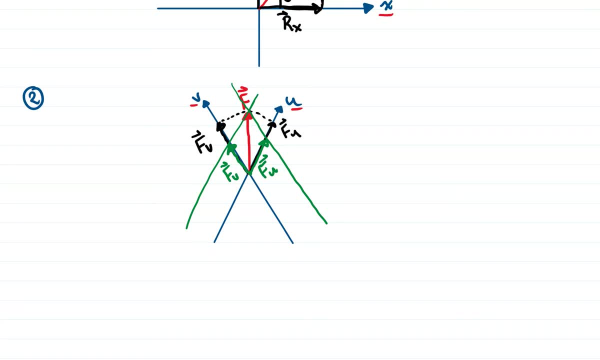 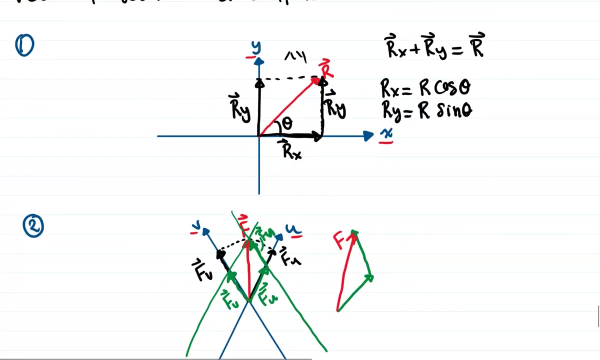 green is also called the vector component. so when we use the head-to-tail fashion, this will be the F sobre f V vector. so let's redraw it here. the difference between: to an example one that in this situation we we use these formulas to find our X. 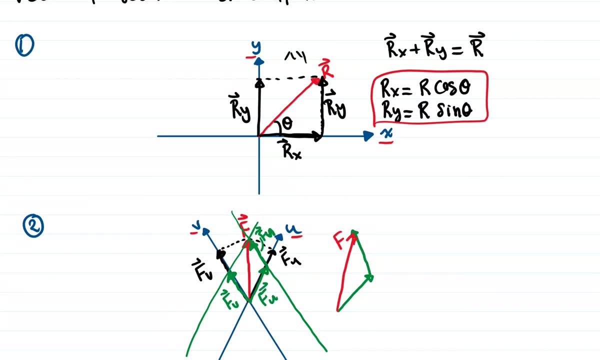 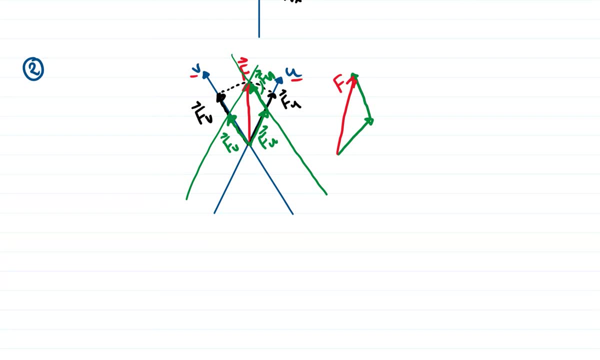 and our Y, because we are dealing with a right triangle in this situation. we are not dealing with a right triangle here. we will deal with the cosine law and the sine law and we will use something called parallelogram theorem, and this is being is being used a lot on on chapter 2 in engineering statics in the problems. 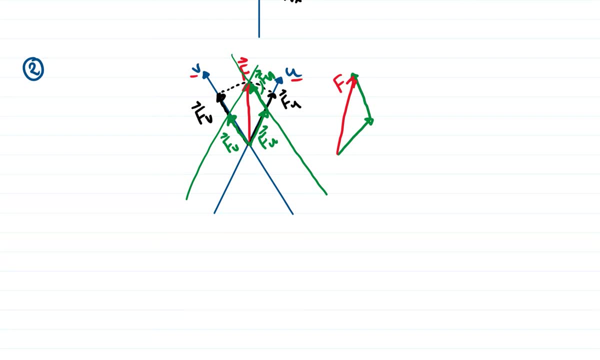 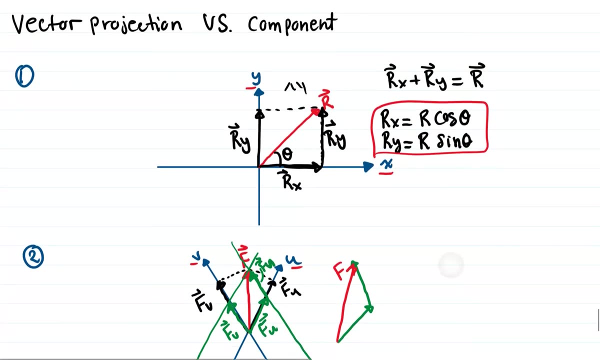 that I already solved and upcoming problems that I will be solving. so that's the difference between vector projection and vector components. if you have any question, please leave them on the comment below and I will make sure that I will answer these questions. thank you very much and have a good day. 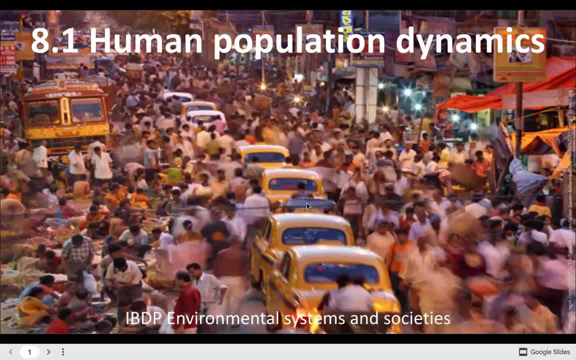 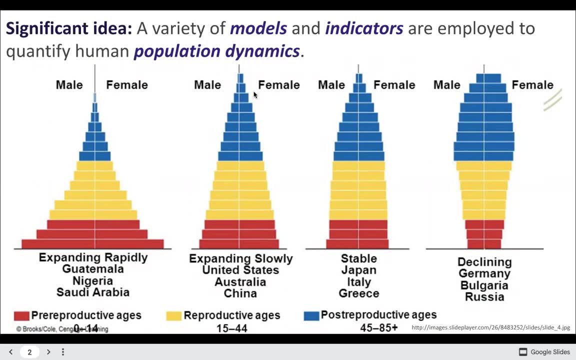 8.1- human population dynamics. So the first significant idea is that we have a lot of models and indicators to study how our populations are changing through time. So here we see males and females, and then their respective ages, in expanding and stable and declining areas. 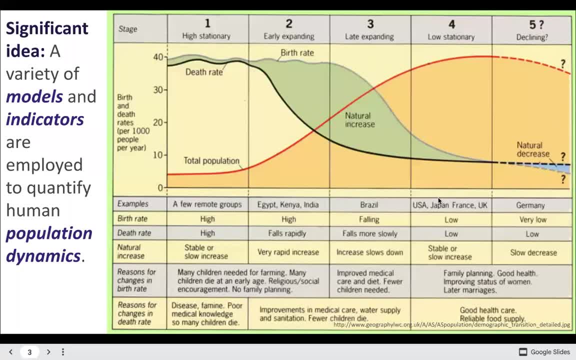 Actually, Japan is over here now. This is an old one, I guess Let's save the date. Another significant idea: Well, here's another model. actually, This is the demographic transition model. So how? population, demographics, birth rates, death rates. 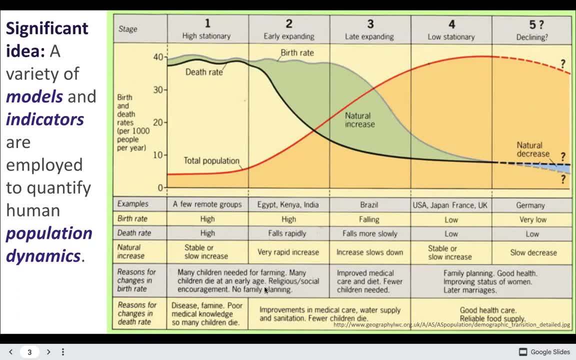 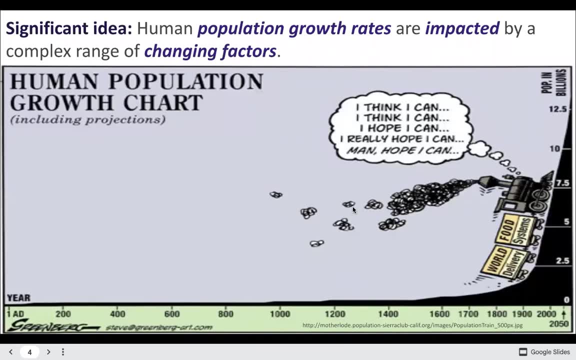 overall population growth change as countries develop and increase their economic security. Human population growth rates are impacted by a complex range of changing factors as we become more intelligent, So we have a lot of data that we can use to study how our populations are changing through time. So we have a lot of data that we can use to study how our populations are. 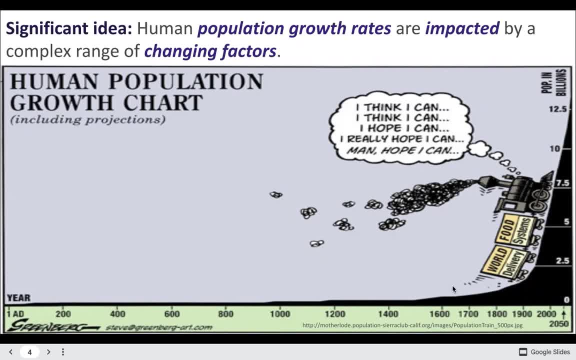 changing through time. So we have a lot of data that we can use to study how our populations are industrialized as we develop more, better food systems. The population of the earth has been skyrocketing. That's pretty wild, Like back in, like what Malthus was like right around here. 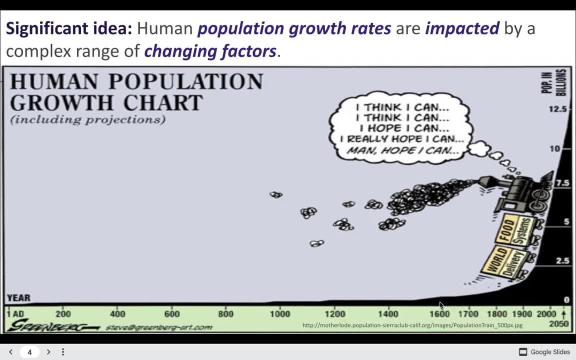 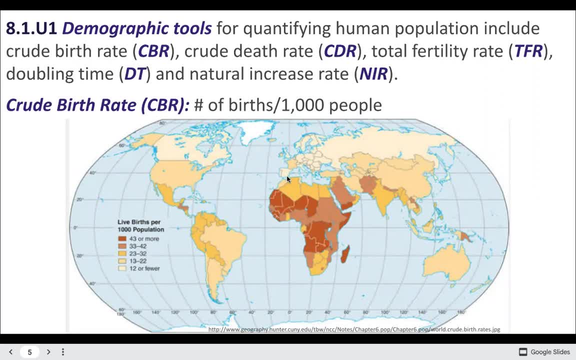 He's like, oh my God, we're not gonna be able to support anyone on earth. And then we're just like: So, first understanding, we got different demographic tools for quantifying human population, And I should have a video where I go through how to do all these calculations. 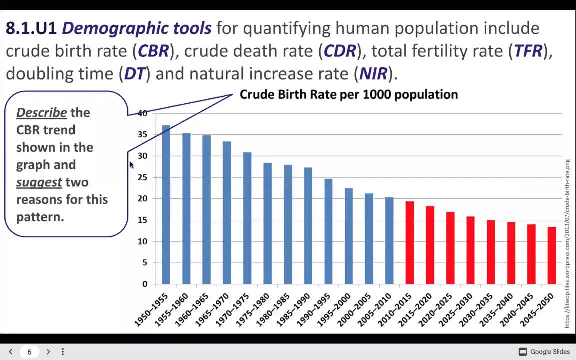 So you can check that one out. Maybe I'll post it in the link. So again, crude birth rate and crude death rate, sort of looking at per total population, Total fertility rate, is looking at births per woman of childbearing age. right, They're the.